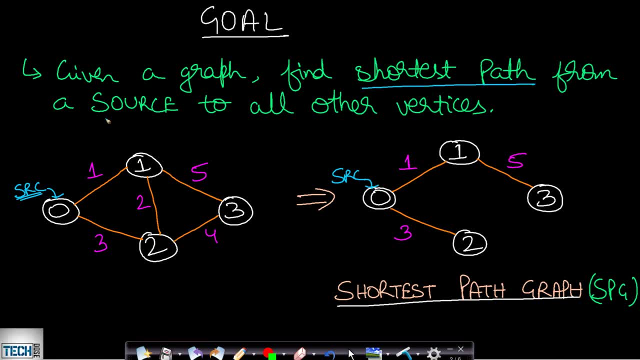 graph and we are required to find the shortest path from a source to all other vertices. let's say this is our given graph and let's say this zero is our given source. now we need to find the path, that is, from this zero to all other vertices. what will be the shortest path? so, from? 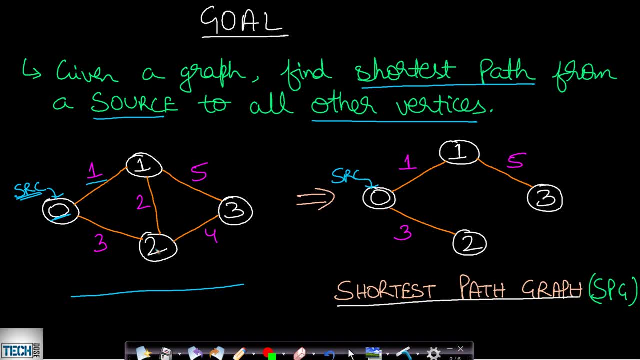 0 to 1. what will be the shortest path? it will be 1, from 0 to 2. what will be the shortest path? there can be two shortest path. it can be 0, 1, 2, or it can also be 0- 2, so we can pick either of them from 0. 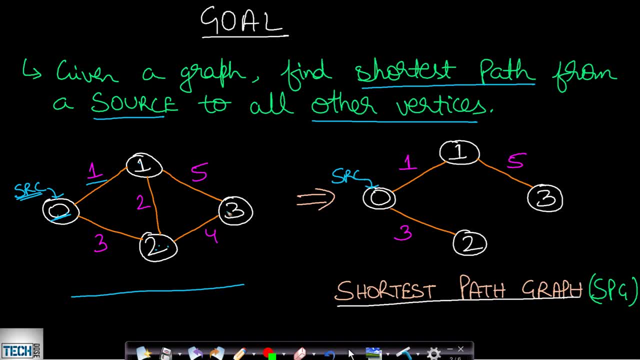 to 3. what is the shortest path? it is 1, 5, which will be 6. okay, so this is the entire problem. we are given a graph and we are given a source and we are required to find, for, starting from this source, what will be the shortest path to all other vertices in the given graph. now, in this, 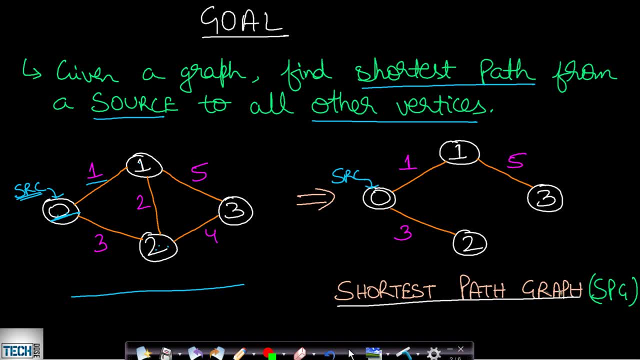 case, i have drawn a possible spg, which is shortest path graph. uh, from 0 to 1, it will be 1. from 0 to 2, it will be 3. from 0 to 3, it will be from 0, 1, 3. okay, so this is one possible spg. now, many of you 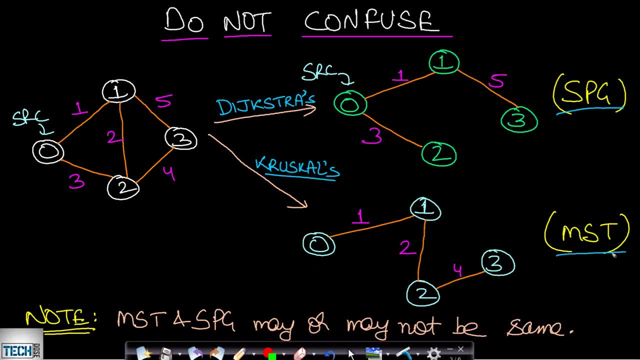 might confuse this shortest path graph with the minimum spanning tree. so i will take the same example and on this graph, if we apply Dijkstra algorithm, then this will be a possible spg- that is, shortest path graph- and if we apply mst, then this will be the possible mst. okay. 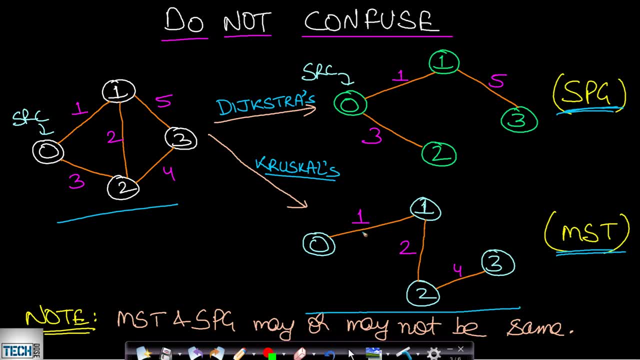 you can see that they both are unequal. so mst and spg may or may not be same, because both these algorithms are different. they have different objectives. okay, so i have already explained this Kruskal's algorithm- i hope you have seen it earlier- and this Dijkstra algorithm. 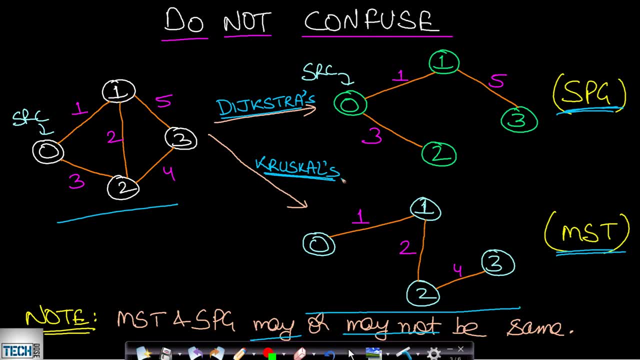 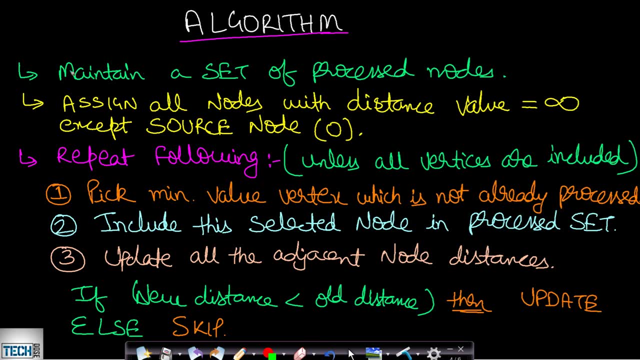 has having a totally different objective as compared to this Kruskal's algorithm. now, coming back to this algorithm, let us see the steps. the steps are very similar to what we did in the prims algorithm, so link to that video will also be present in the description below you can. 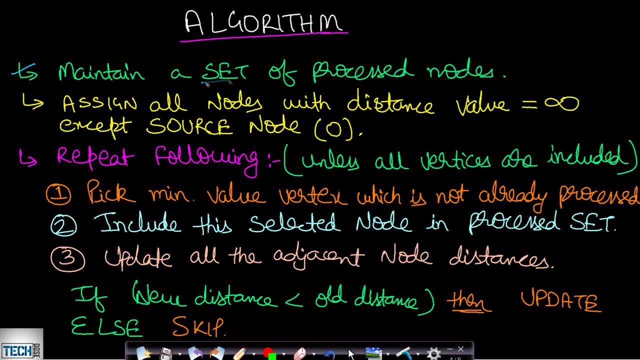 check that out now. the first step is we need to maintain a set which will keep track of all the processed nodes. now the next thing is we will assign all the nodes with the distance value equals to infinity, except the source node, which will be equals to 0. and why is that? because we 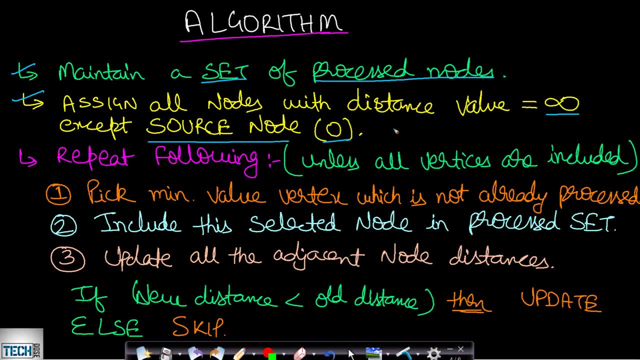 will be picking the minimum value of the distance node and we will be picking the minimum value of the node and we will try to process it so when all the nodes are made infinity except this source node, then this source node will be picked first, because this is having minimum value, which is 0. 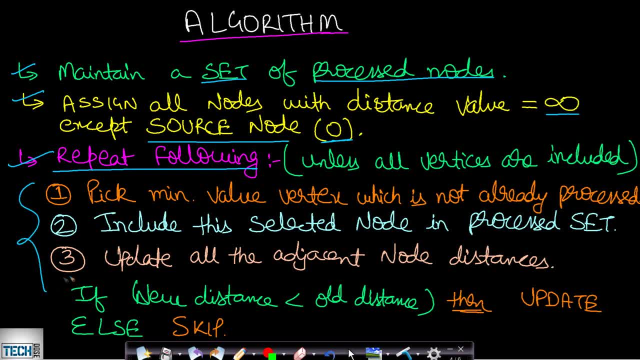 so we will have to repeat these processes unless our graph is finished, unless we have formed our spg. so the first step is we need to pick the minimum value vertex, which is not already processed. so the first time we will be picking this source node, because all the other nodes will be having infinity value. 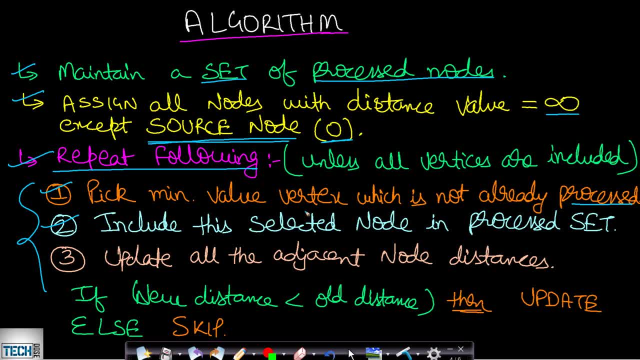 now the second step is include this selected node in the processed set. so whatever node is getting selected, we need to mark it as processed. now our third step is to update all the adjacent node distances. so let's say we started from this zero, we were at one, and now from one we are having two. 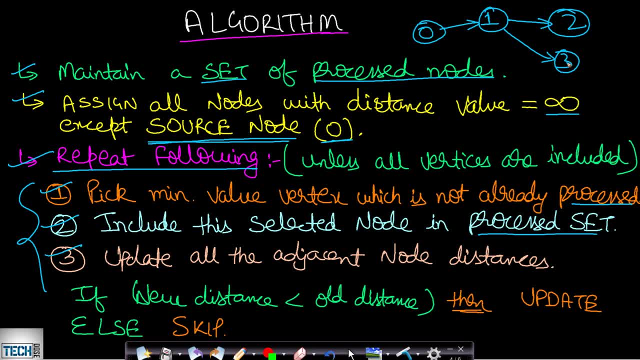 adjacent nodes which are two and three, let's say, to this three there was another path through this four. okay, so what can happen is, let's say its distance was one and now we have two adjacent nodes because the distance was one and three. then the distance to this three from this zero would have. 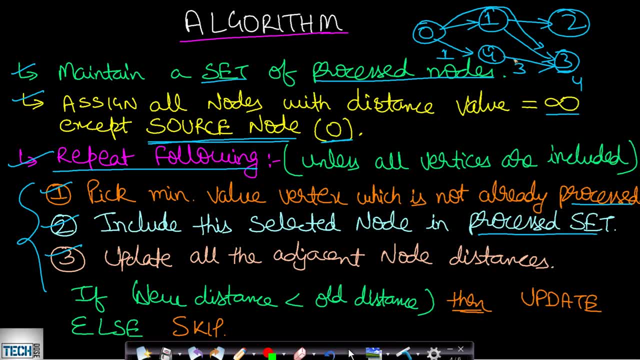 been four and now, since we are passing through this one, then the distance might be different and it might be lower than the already calculated distance. maybe the distance here was one and it was also one year. so now, through this path, if we use this one, then from zero to three we can reach. 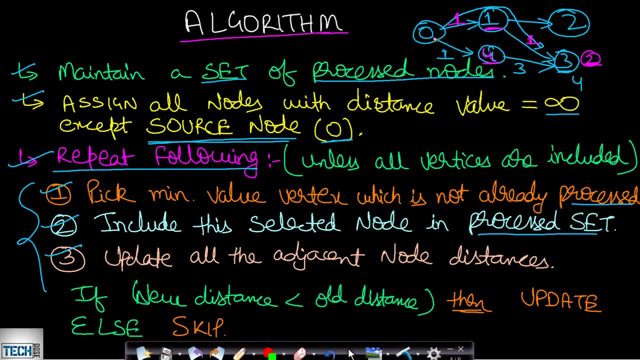 at a cost of two. but we had calculated earlier that if we use this node four and move from zero to three, 4, so we need to update this value 4 to a lower value, since we want to find the minimum cost in order to start from this source node and reach to the given vertex. okay, so that is why we will. 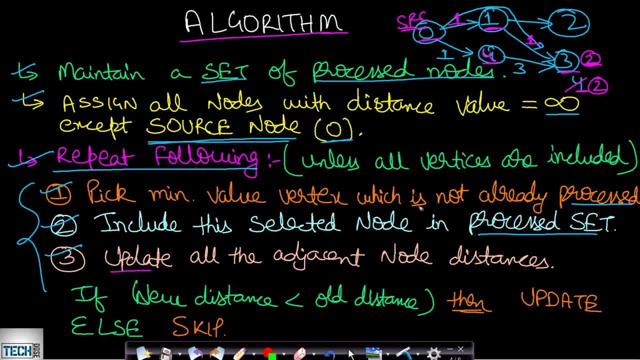 update all the adjacent node distances, and the update criteria will be: if the new calculated distance is less than the old distance which is already given, then we will update. otherwise we will skip updating. okay, so these will be repeated unless and until all the v vertices have been. 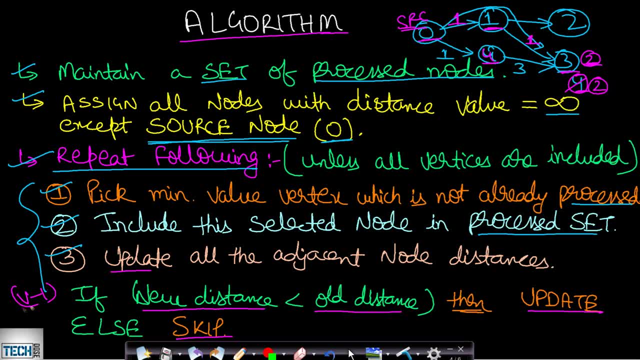 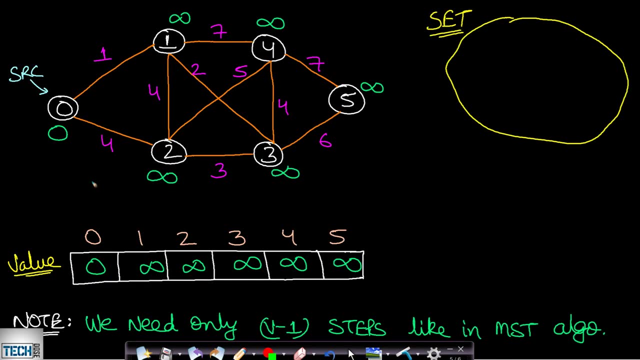 covered. so in this algorithm as well, we need to process v minus one times, like we did in mst, because we have v vertices. so we will be having v minus one number of edges in this spg as well as in mst. let us now look at an example in order to get a better understanding about this algorithm. 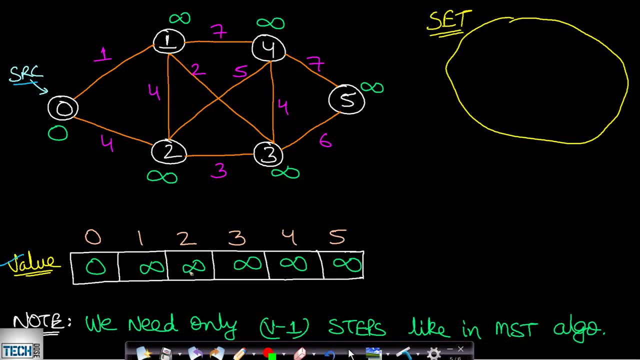 so we are given a source node and i will be taking a value array here. the source node will be having value zero and all the other node values will be infinity. so initially, r4 step was to pick the minimum value vertex. so we will pick the minimum value vertex, which is zero. 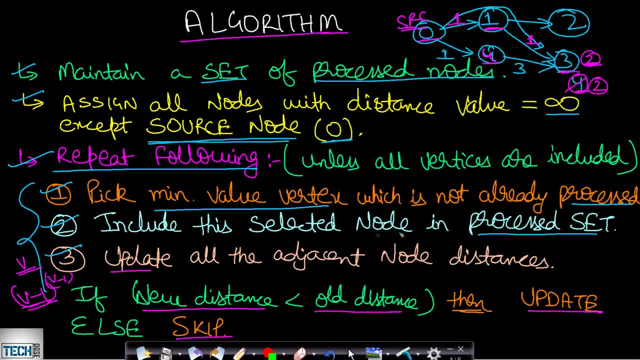 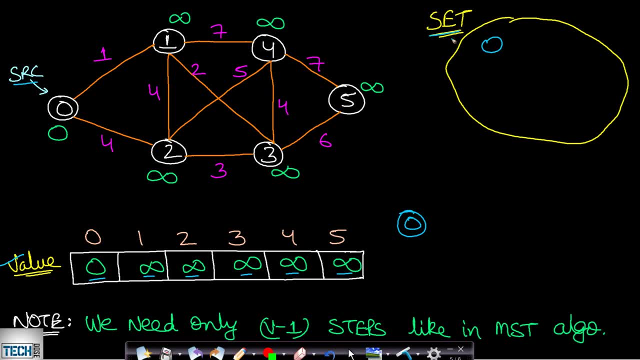 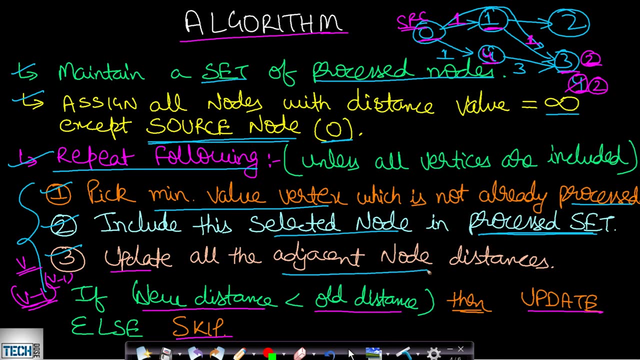 so zero will be picked now. our second step was to include this selected node in our processed set. so we will include this node in our processed set, so this will keep track of what all nodes have been processed, so that it doesn't get processed again now. the third step was to update all the adjacent 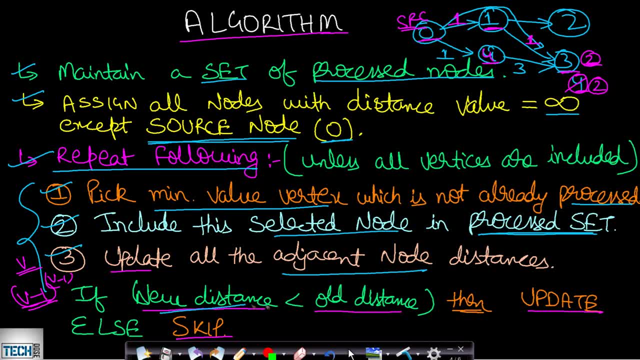 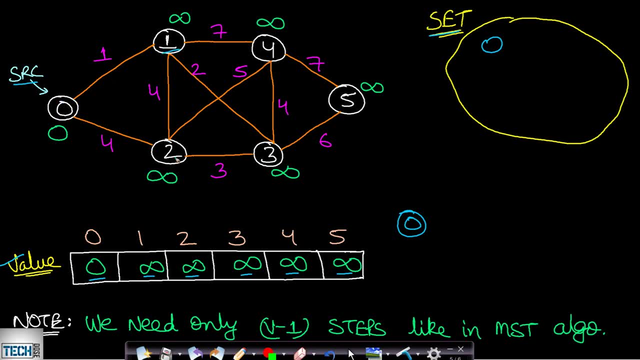 node and the updation criteria was: if the new distance is less than the old distance, then we will update, otherwise we will skip. so what are the adjacent nodes from zero? adjacent nodes are one and two. what are the already present values from zero? if you see this one, then the cost will be. 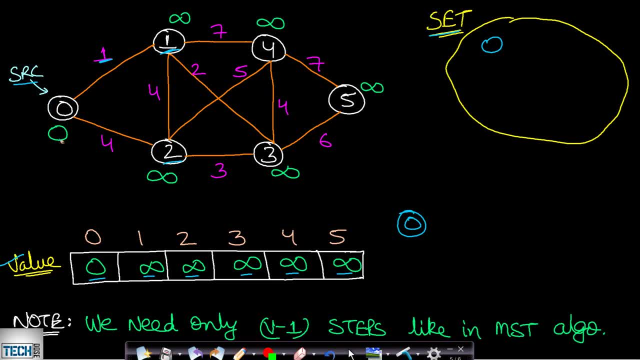 cost at 0 plus this edge cost. so the cost at zero is 0 and the edge cost is one. so if you add zero to one, then this will be one. so what will be the minimum of this one comma infinity? it will be one. so this infinity will now be replaced by one. okay, and how do you update this node too? it is having 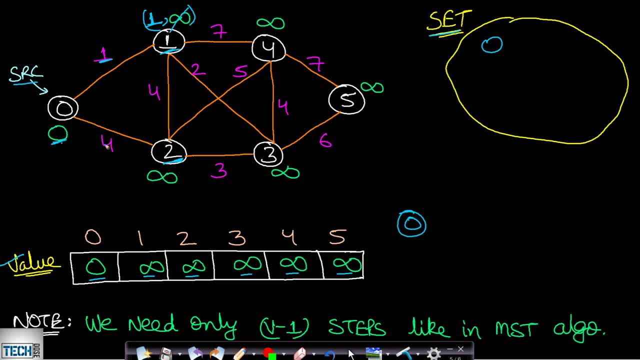 value infinity, but the new cost is 0 plus 4, which will be equals to 4. so if you take minimum of this 4 comma infinity, then that will be 4, so we will update this infinity with 4. okay, so this is how updation is done, and now this node 0 is processed. so what will be the next node which we need to? 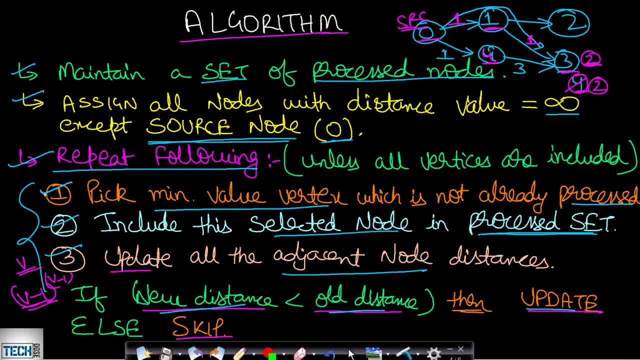 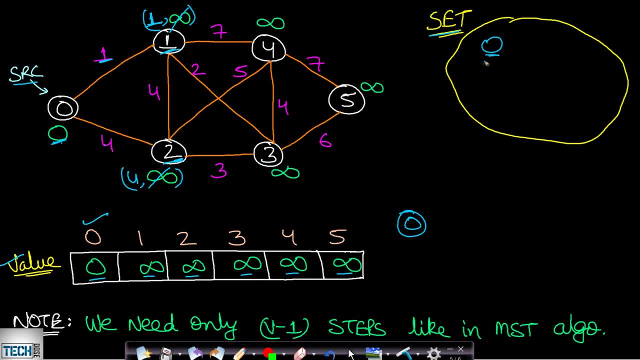 process. we will have to again repeat these steps. so we will again go to this step one. we will pick the minimum value vertex, which is not already processed. so this 0 has already been processed, so we cannot choose this now. the value of this one, that is, cost of 1, is 1 and cost of 2 is 4. 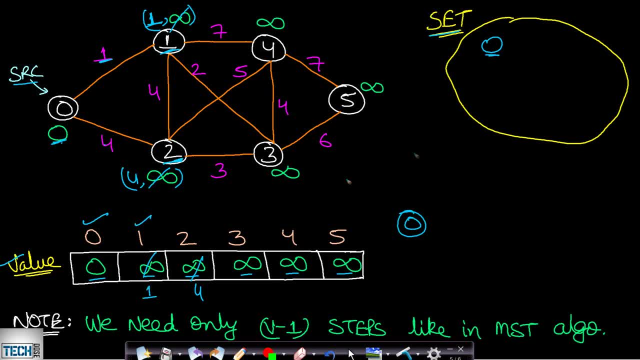 so the minimum value is this: 1. okay, so 1 will be picked and this will be included in our processed set. and now all the adjacent vertices of 1 will now be relaxed. now you cannot relax an already processed node, so 0 will not be relaxed from 1, the distance to 2 will be cost of 1, which is 1. 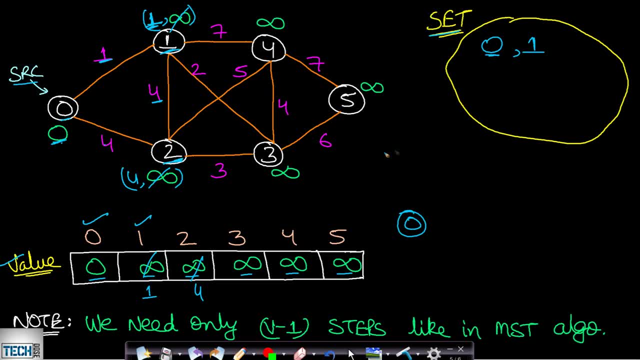 plus this 4, which will be equals to 5.. so minimum of 5 comma 4 will be nothing but 4. so this will not get updated from this one. the distance to 3 is cost at 1, which is 1 plus this 2, this will be equals to 3. so minimum of 3 comma infinity is 3. 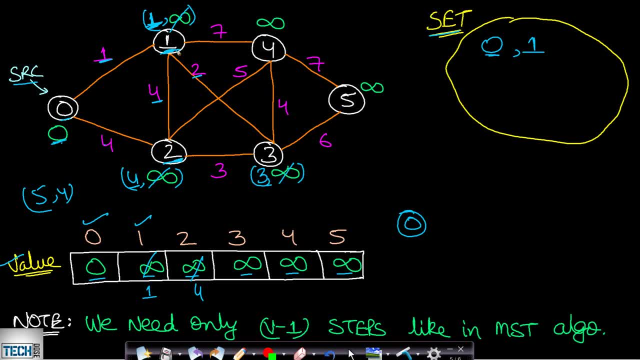 so infinity will now be replaced by 3.. now the distance from 1 to 4 will be minimum of the cost at 1 plus 7 comma, this infinity. okay. so 1 plus 7 comma infinity. so this will be 8. so infinity will. 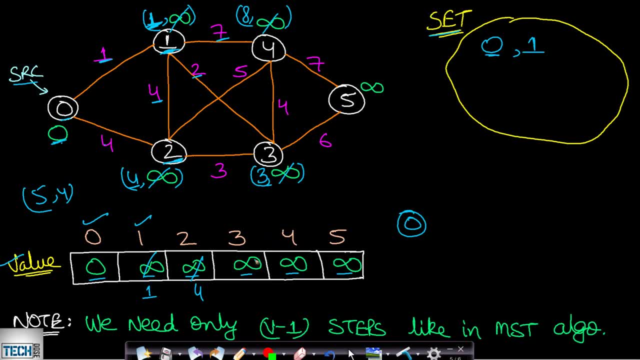 now be replaced by 8.. let me also update this in our value array. so 3 will now be updated to value 3 and 4 will get updated to value 8, and now 1 has now been processed, so 1 will get included. 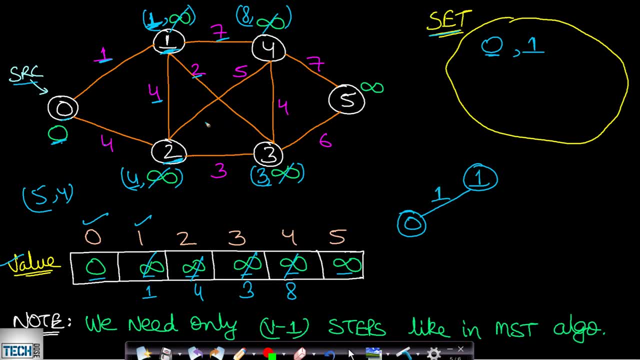 the edge weight is 1. okay, and now we will again move back to the first step. so what was the first step? our first step was to include the minimum value node, which is not already processed. so 2, 3, 4, 5 nodes are not processed. so the minimum distance node is this: 3. 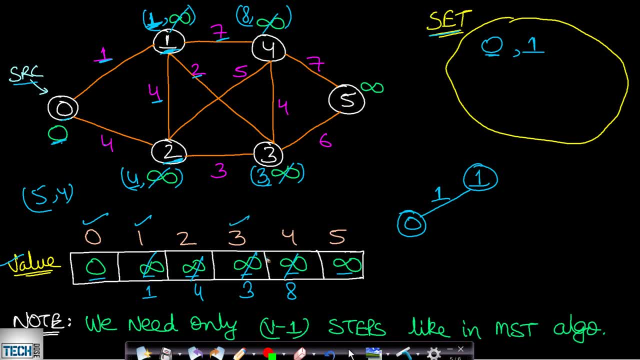 so the minimum distance node is this 3. so we will pick this 3 because this is having minimum cost, which is 3.. so 3 will now be marked as visited, that is, as processed. and now we will go to this 3 and relax all the adjacent vertices. 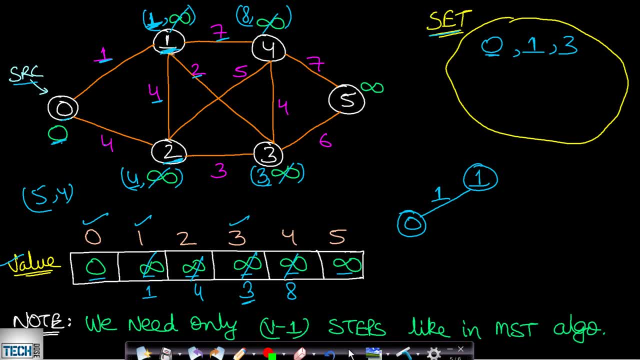 so from this 3, you cannot relax this 1 because 1 is already processed now. from this 3, the distance to 2 will be 3 plus 3, which will be 6, but already present distance is 4, so 2 will not be updated. 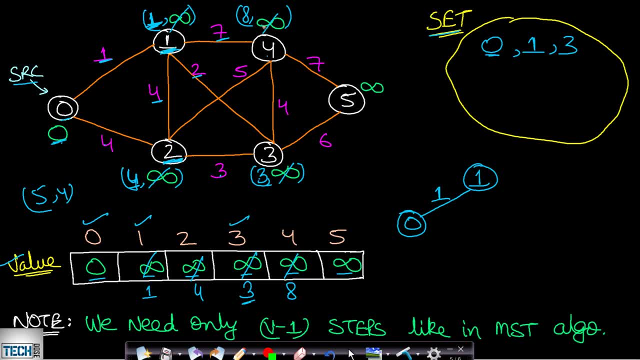 now from 3, the distance to 4 is 3 plus 4, which is 7. so we will take minimum of 8 comma 7, which will come out to be 7. so you can see that we have found a new minimum cost path to this 4, starting from this 0 which is going via this 3, so already found. 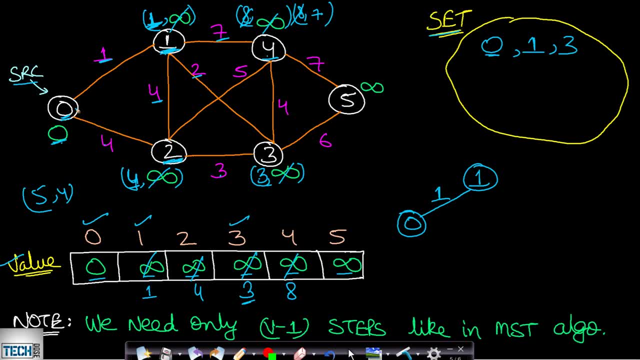 path was having cost 8, which was through this 1, which was 0, 1, 4. but now, when we have included this node, 3, then the new minimum distance is 7 and this is 0, 1, 3, 4. okay, so we will update. 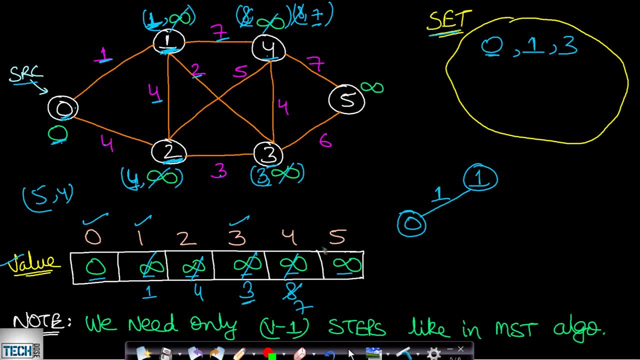 with this new value and let me also update this here. this is 7.. now from 3 the distance to 5 will be 3 plus 6, which is 9. so minimum of infinity comma 9 will be 9. so it will get updated to value. 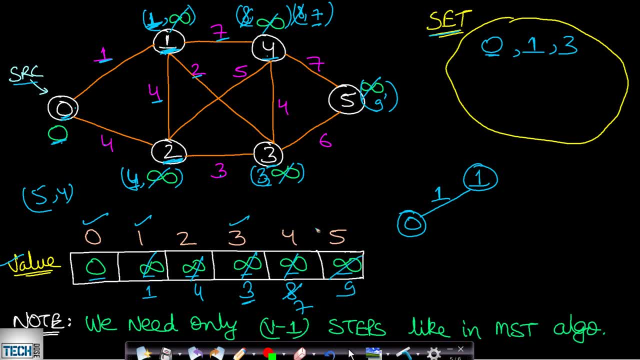 9.. now 5 will have value 9. and now we will again move back to the first step. so our first step was to pick the minimum among the unprocessed nodes. so one process node is 2, 4 and 5.. which node is having minimum value? this will be 2.. 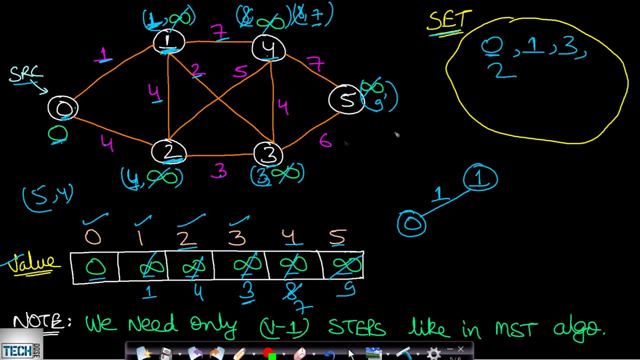 we will pick this node 2, we will mark it as visited. and from 2 you cannot relax this node 0 because this is processed. you cannot relax this node 1 and node 3 because they both are also processed now. from 2 you can try to relax this 4, so cost of 2 is 4. now, if you want to calculate, 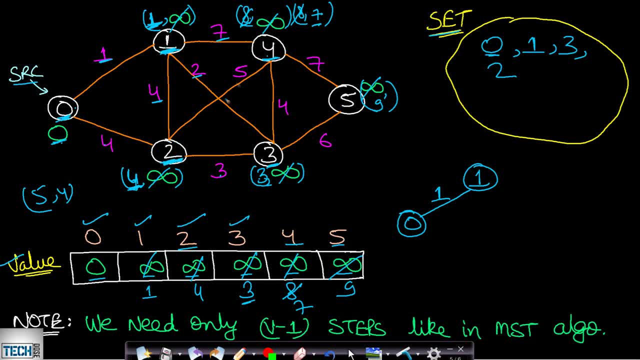 the minimum cost starting from this source, going via this 2 to this 4, then the cost will be the cost to reach this 2, which is 4, plus the edge weight that is cost to reach to this 4 from 2. so this will be 4 plus 5, which will be 9. but the already present cost is 7, which is lower. 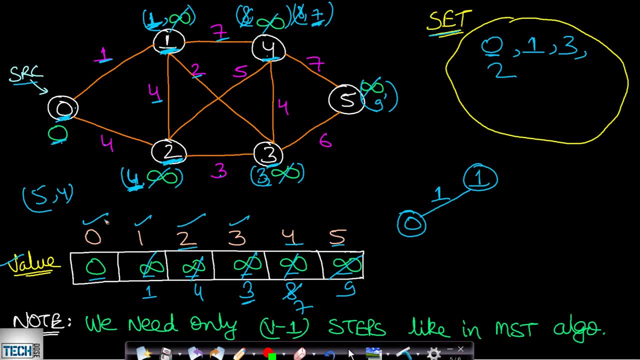 so we will not update it now. 2 has now been processed and we are done with the three steps. now we will again repeat the step, so we are left with only two nodes. so let me also update the spg graph. after one, we had selected this node 3 having weight 2, and then we had selected this: 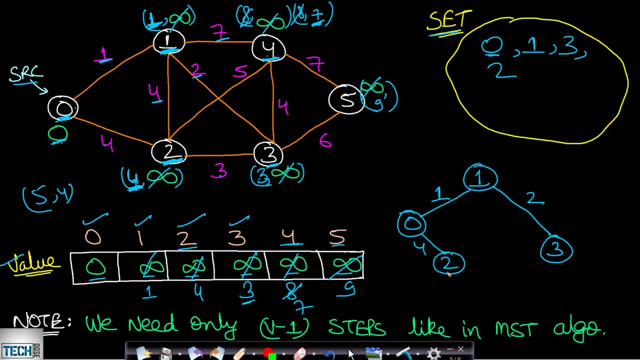 node 2, having this weight 4.. now, after selecting this node 2 again, we will perform step one. we will pick the minimum weight node, so the minimum cost node is: this is 4. so 4 will get selected. we will include it in our set. that is our processed set and now we will try to relax all its adjacent. 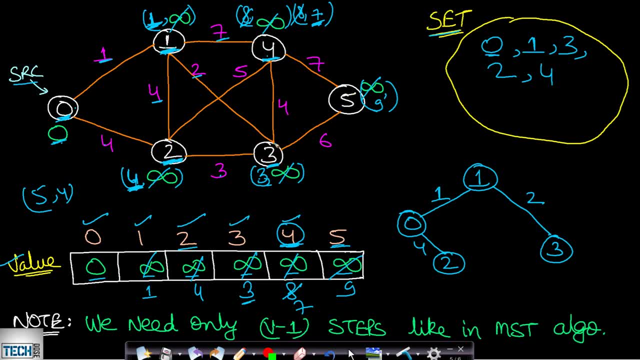 vertices one, two, three are already relaxed, so we will try to relax this five now. the minimum cost in order to reach this four from zero is equals to seven. okay, and now from four to five, you will require cost at four plus this cost, which is seven. so seven plus.